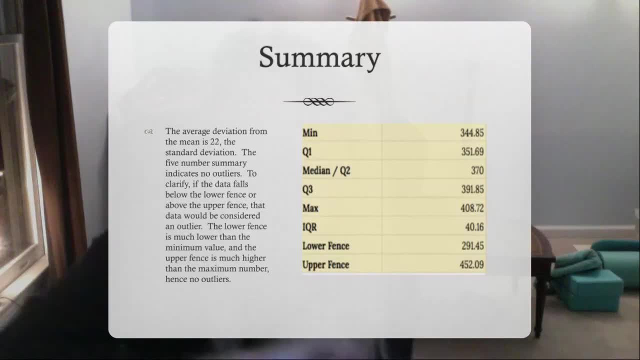 We also have the five-number summary here. This indicates no outliers. so to clarify if the data falls below the lower fence or above the upper fence, that data would be considered an outlier. So if you look here, you can see that the data falls below the lower fence or above the upper fence. 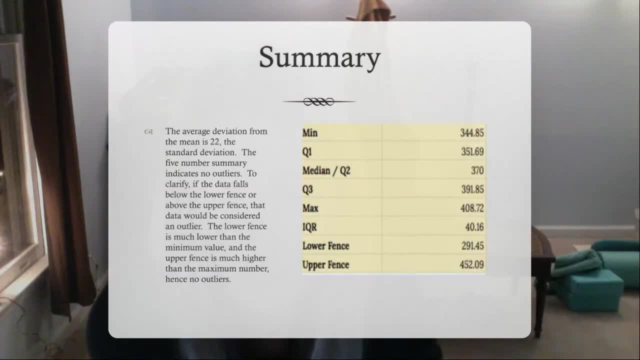 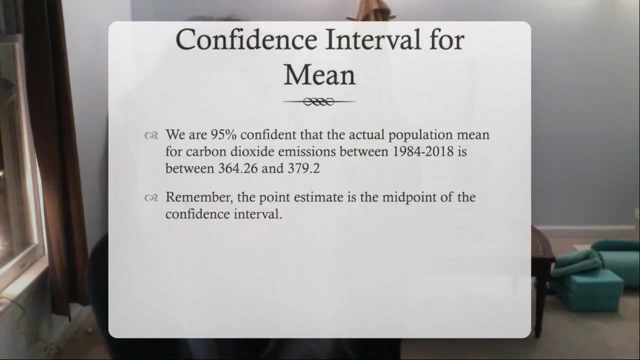 So if you look here, you can see that the data falls below the lower fence or above the upper fence. So if you look at the lower fence, it's much lower than the minimum value, and then the upper fence is much higher. So no outliers here. 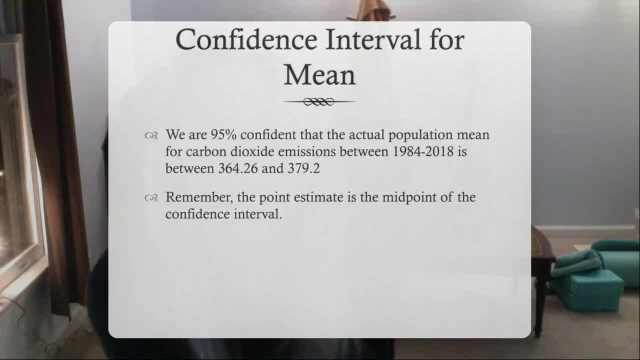 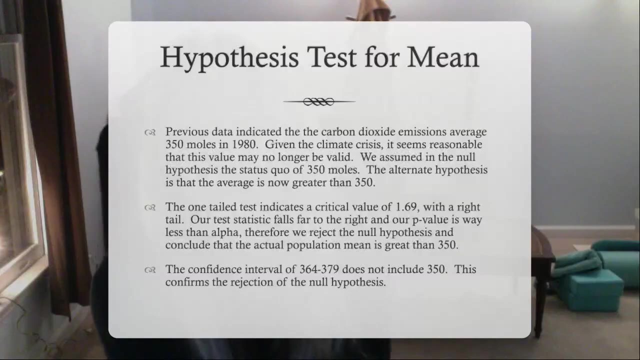 Our confidence interval. so we are about 95% confident that the actual population mean for carbon dioxide emissions between 1984 and 2018 is between 364 and 379.. We did a hypothesis test for a mean So you can see here: the population mean for carbon dioxide emissions between 1984 and 2018 is between 364 and 379.. 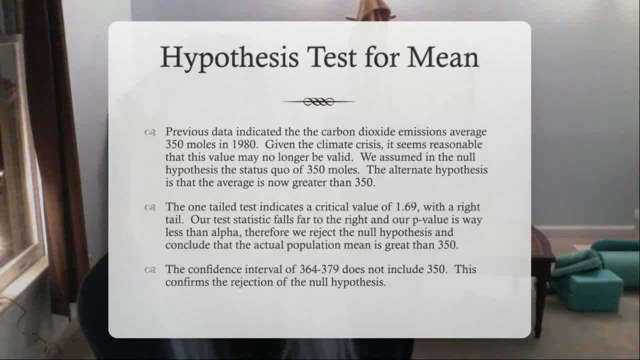 The previous data indicated the carbon dioxide emissions averaged 350 moles in 1980.. Given the climate crisis, it seems reasonable that this value may no longer be valid. We assumed in the null hypothesis the status quo of 350.. The alternate hypothesis is that the average is now greater than 350.. 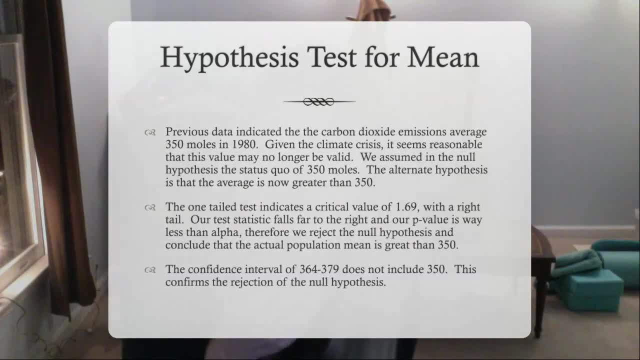 The one-tail test indicated a critical value of 1.69, with a right tail Our test statistic falls far to the right in our p-value. So that's when we figured out that 15,000 moles, or probably 20,000 moles, would fit between 325 and 350.. 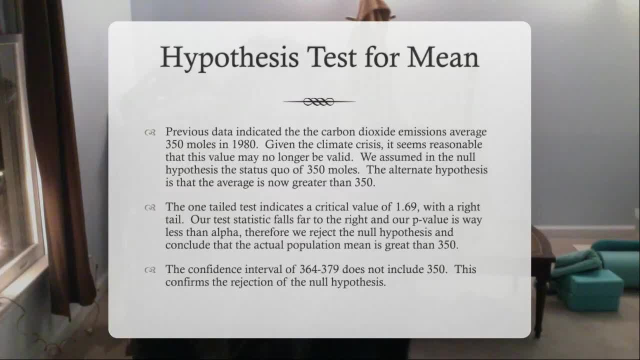 is way less than alpha. Therefore we reject the null hypothesis and conclude that the actual population mean is greater than 350.. So the confidence interval of 364 to 379 does not include 350.. So this right there confirms the rejection of the null hypothesis. 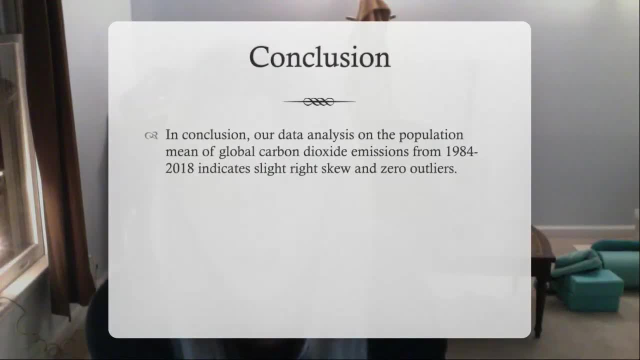 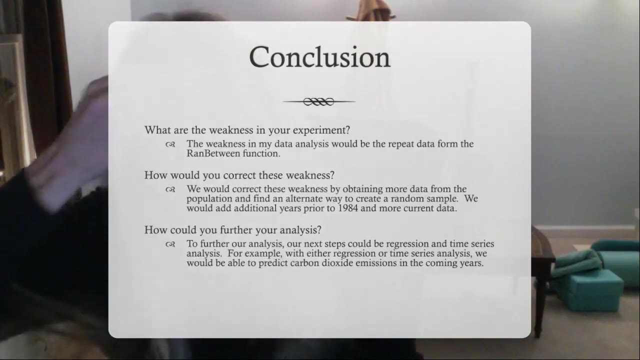 So, to conclude, our data analysis on the population mean of global carbon dioxide emissions from 1984 indicates a slight right skew and zero outliers The conclusion. So there looks like there's some questions here. What are the weaknesses in your experiment? So, probably just the ran between function and some of that repeat data. 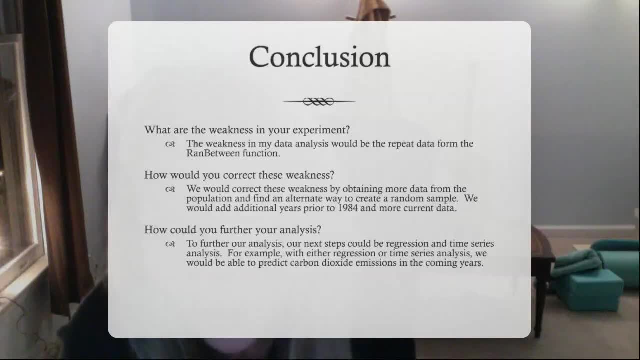 We could correct those by finding an alternate way to create a random sample. We could also add additional years prior to 1984 and maybe some more current data. How would you further your analysis So we could do a regression and time series analysis?